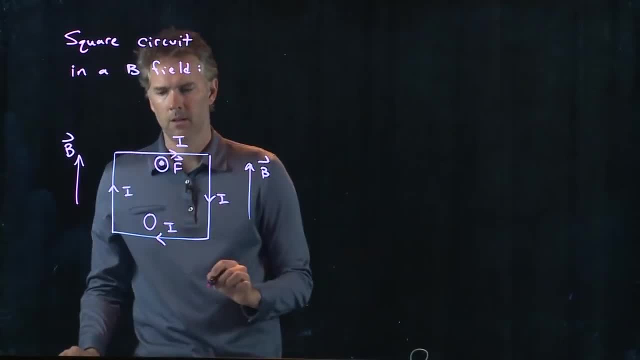 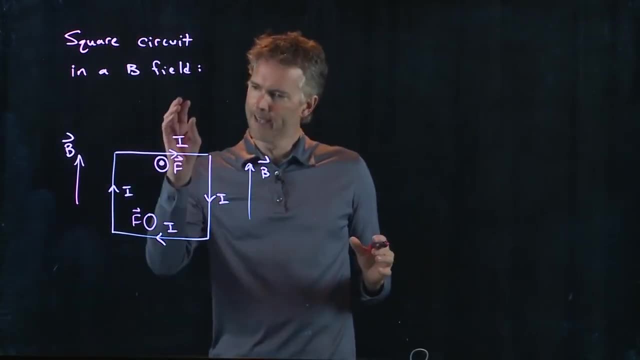 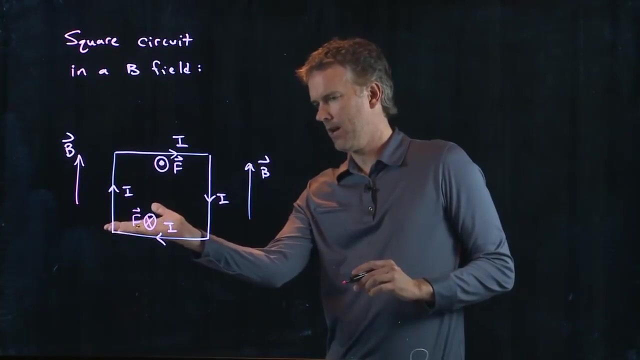 Good, What about this side? The force on this side has to be just the opposite of what we just did. right, We got a dot. This one has to be an X. Let's just confirm I is going to the right. 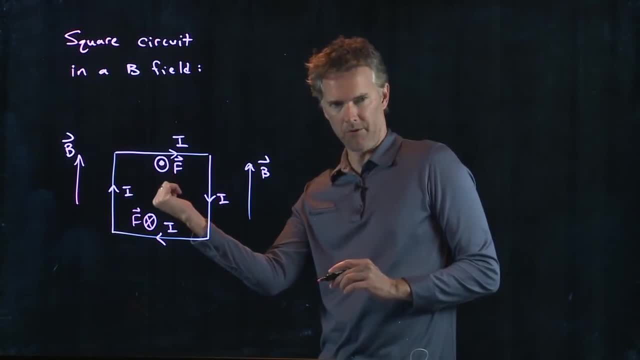 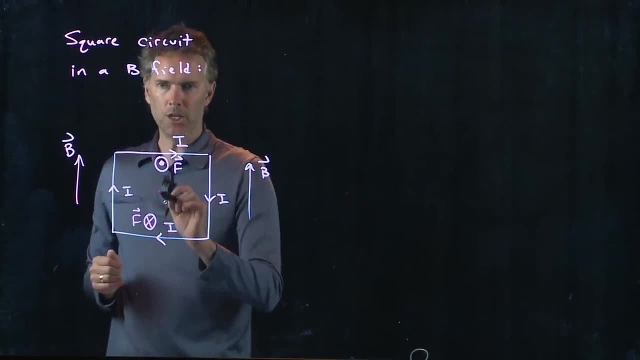 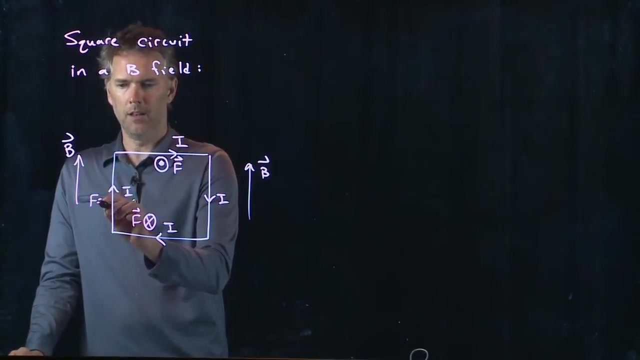 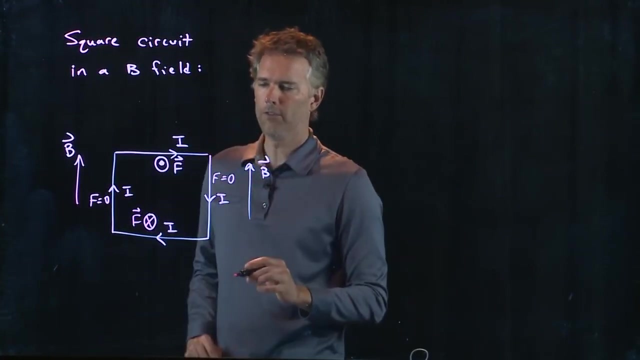 B is going up, My thumb is going into the screen. okay, And so you get a force that is right there with an X into the screen. What about the force on either side? The force on this side is, of course, zero because they're parallel. The force on this side is also zero because they're anti-parallel. 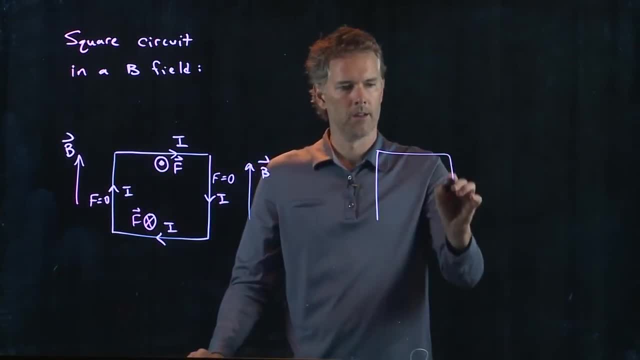 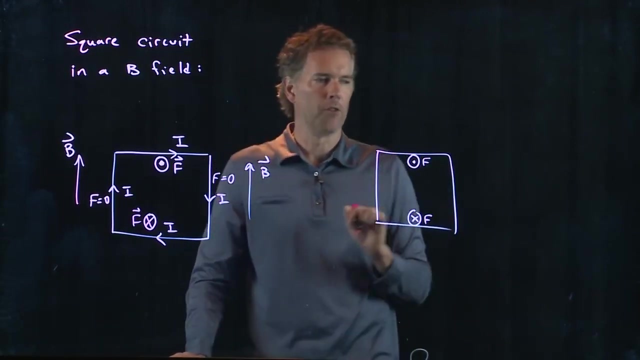 And so that entire square looks like this: It's got a force up here that's going in, It's got a force down on that side that is going out. Sorry, out of the screen, into the screen, And so the net force. 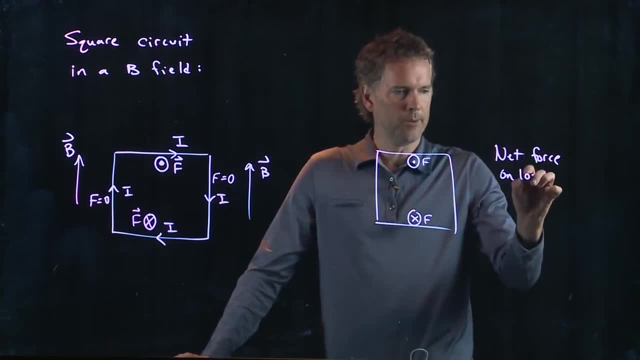 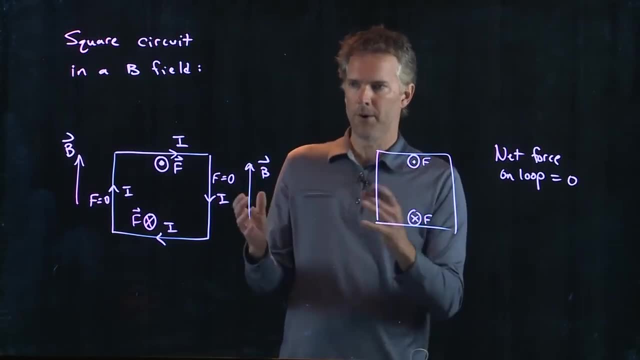 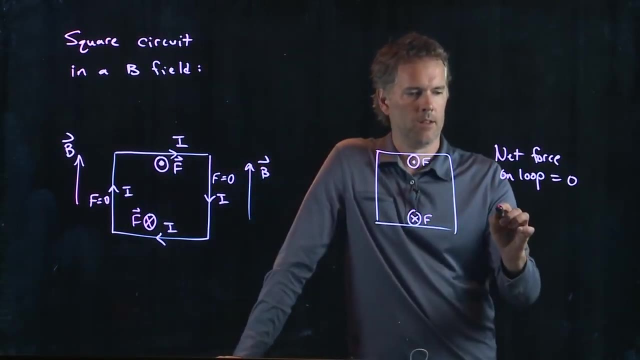 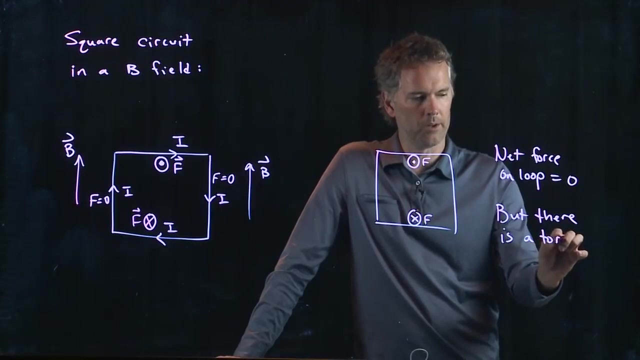 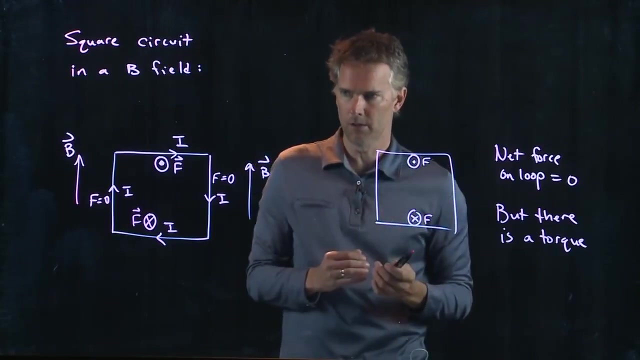 on, this whole loop is equal to zero. Okay, The whole loop doesn't move up or down, or left or right, but there is a twist, There is a torque, because one side is trying to come out of the screen. the other side is trying to go into the screen. 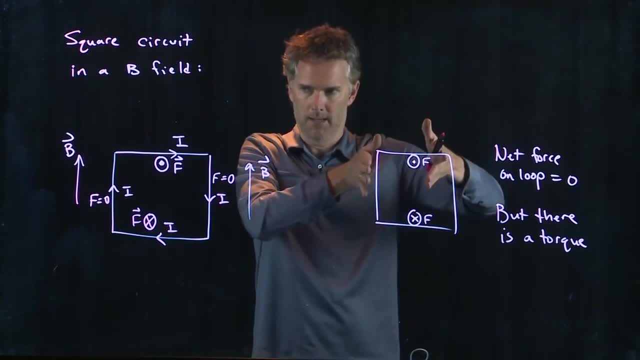 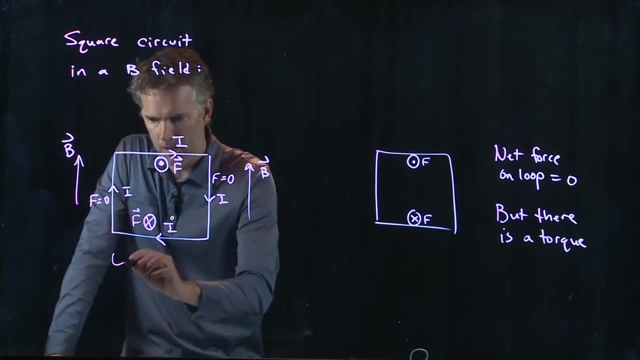 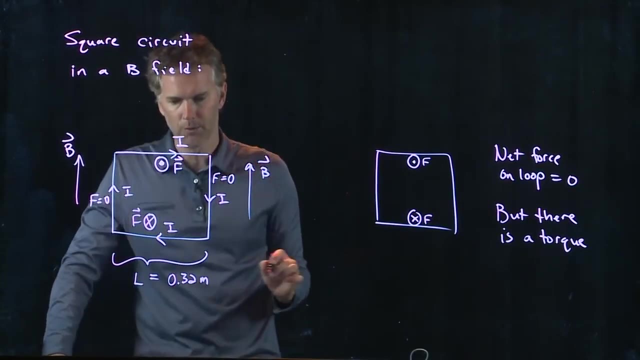 And so this entire thing is going to rotate in this B field. Let's try it with some numbers here and see if we can calculate what's happening. This is a square of side L, and let's say it's 32 centimeters, which is 0.32 meters. 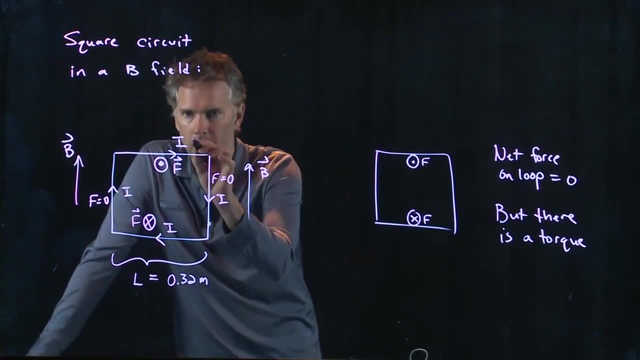 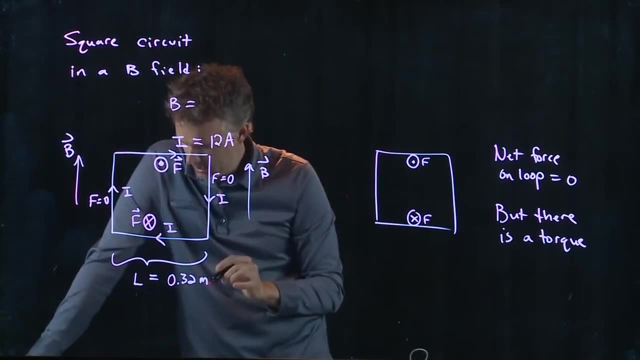 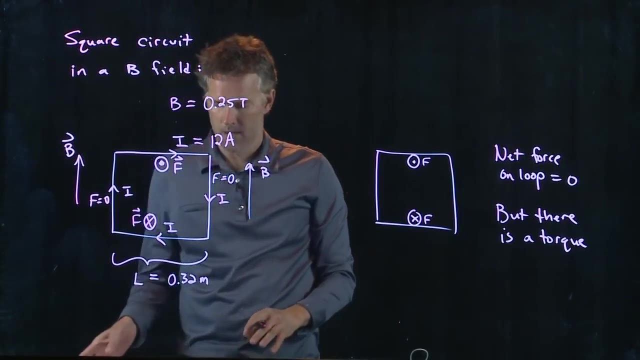 Let's say that the current running around in this thing is 12 amps And let's say that the B field that it's sitting in is a quarter tesla. All right, Let's do each side individually and calculate the force on it. 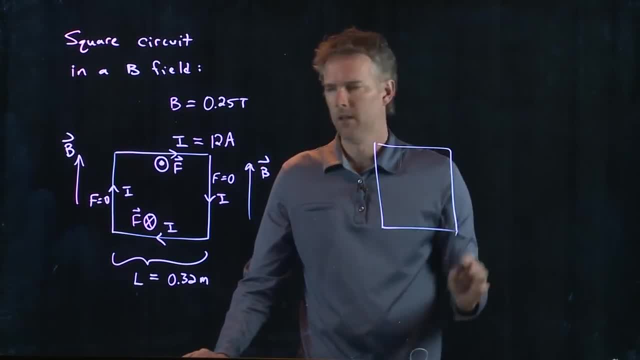 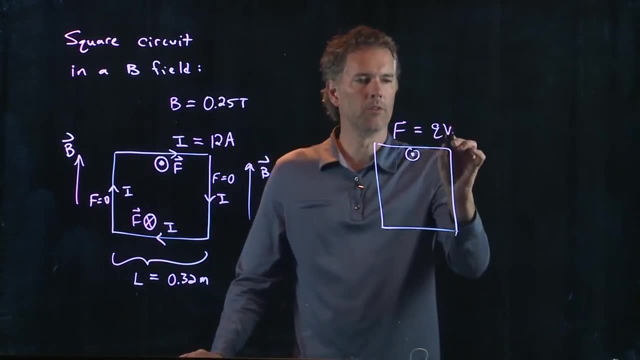 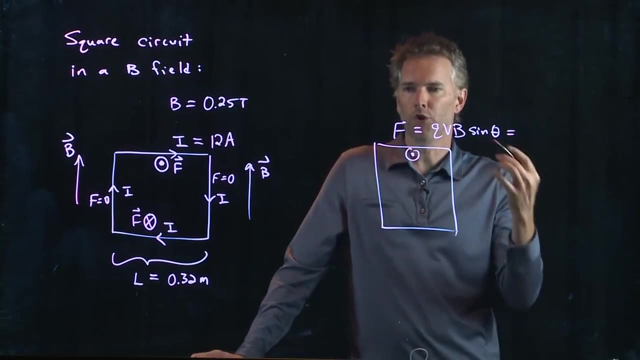 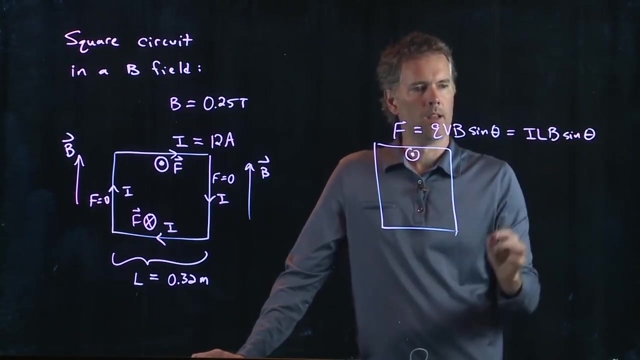 So the top side. we said there is a force coming out of the screen and that force is going to be QVB. So that's going to be QVB sine theta. okay, but we know that QV turns into IL. We give you I, we give you L, we give you B. What is the angle between those two? 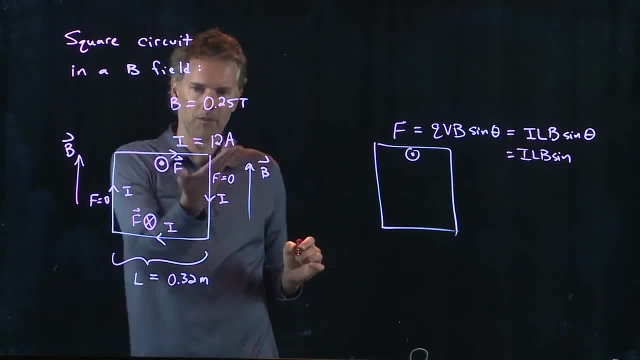 Well, I was to the right, B was up. Those are 90 degrees to me. So that's going to be QVB sine theta. but we know that QV turns into IL. We give you I, we give you L, we give you B. What is the angle between those two? 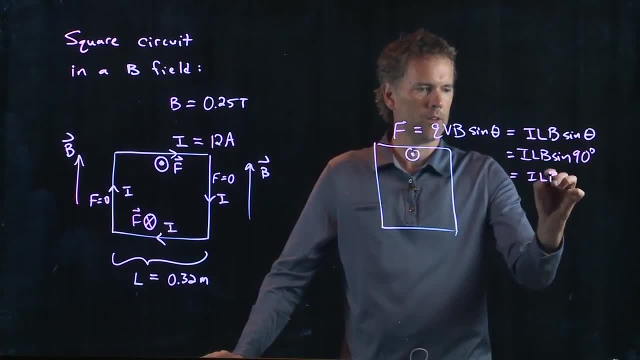 Well, this side turns into IL, So that's going to be SI units. So that's going to be SI units. L is a small amount of time, but if we make that into IL we get what we want And we can do the recovery function. 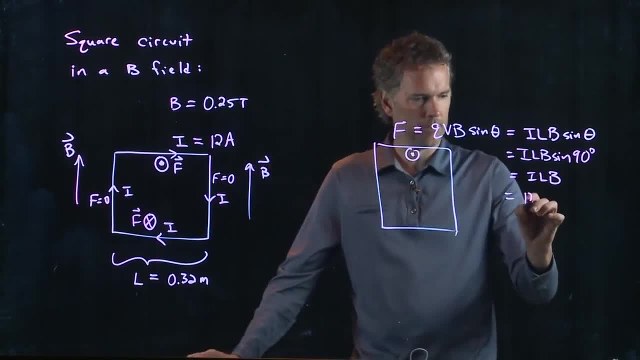 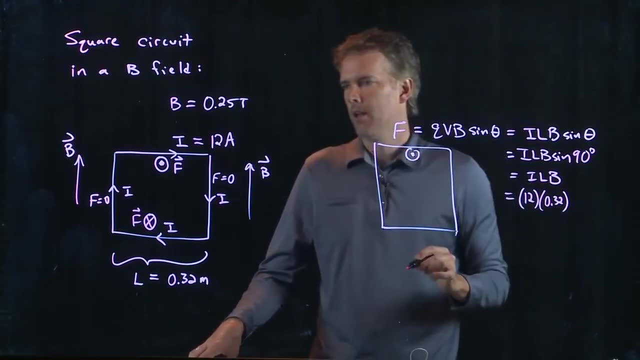 So we get ILB, We get the SI units. We maintain that. And if we multiply the sine of 20, we get the SI units. If we multiply the sine of 90,, we get ILB, And we know that those numbers are actually the same numbers. 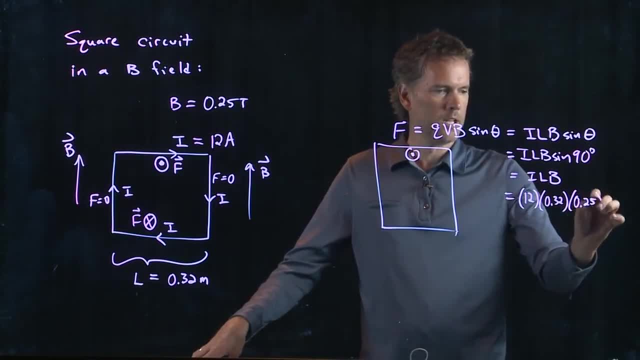 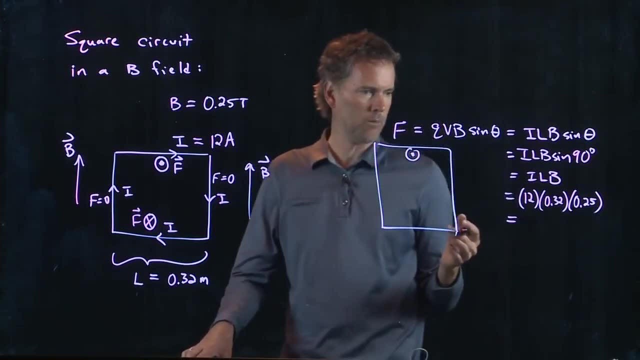 We get the ILB, And so we get 1.. And so we get ILB. And we know what those numbers are. I is 12 amps, That's SI units. L is 0.32 meters And B we said was 0.25 tesla. 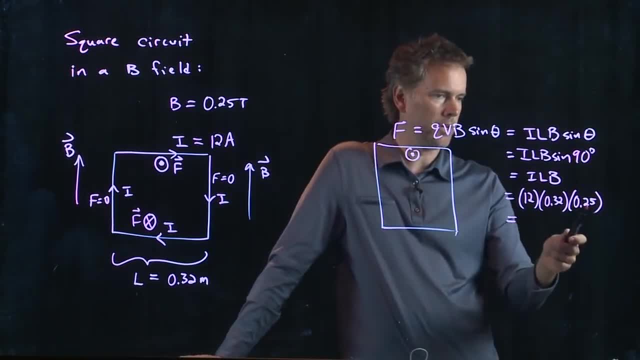 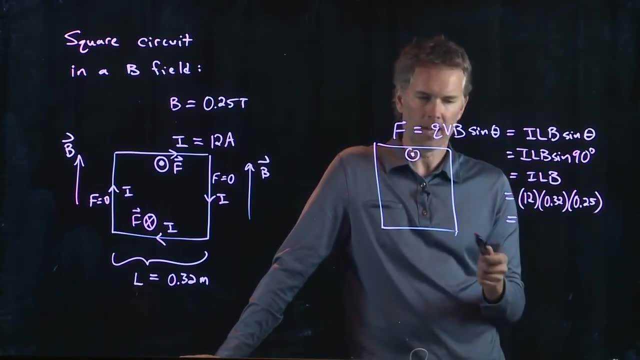 Okay, And let's run those numbers and see what we get. punch it into your calculator and tell me what you get. I'll approximate it here. We got a quarter of 12.. A quarter of 12 is 3.. 3 times 0.32 has got to be really close to 1.. Maybe it is more like 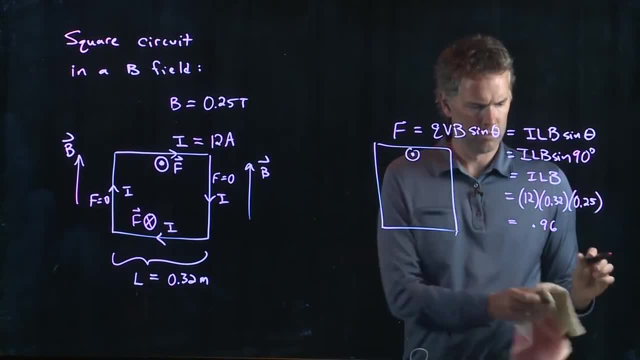 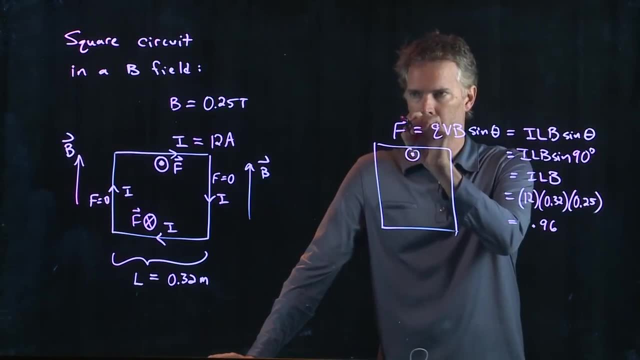 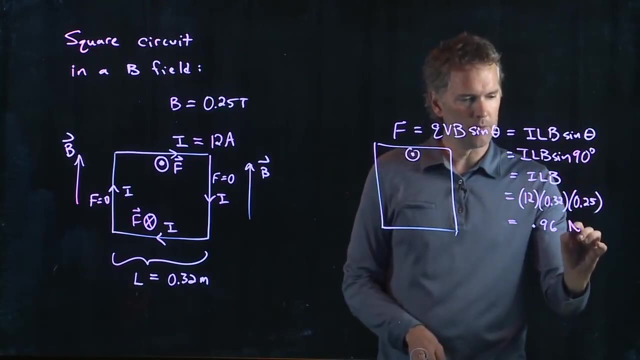 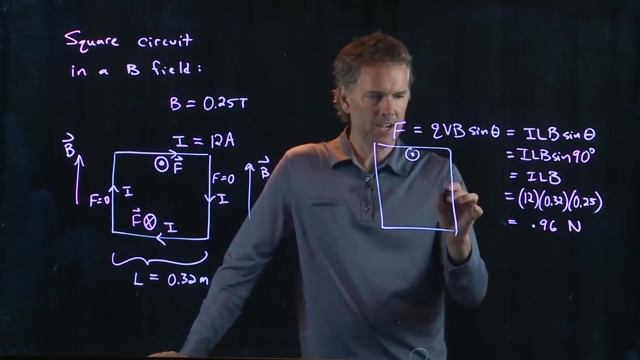 0.96.. Is that what you get if you plug it into your calculator? Okay, 0.96.. And it's a force, right? So these SI units, amps, times, meters, times Tesla gives you newtons. That's the force on the top wire. The sides, we said were 0. So we don't have to worry about. 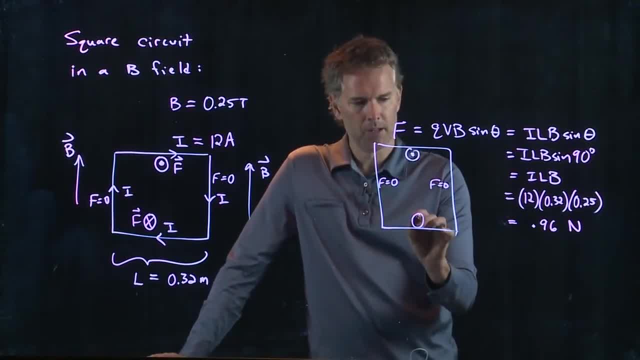 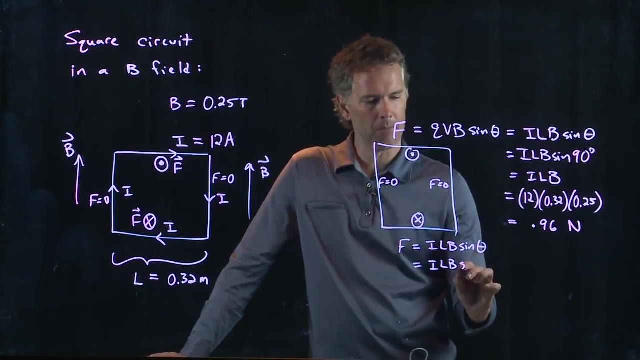 those. The one on the bottom is into the screen And guess what? That's going to have the exact same strength As the one on the top, Because it's a square wire. it's the same length. We have the same angle. 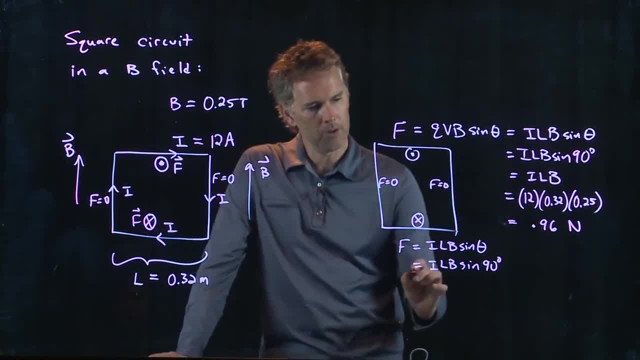 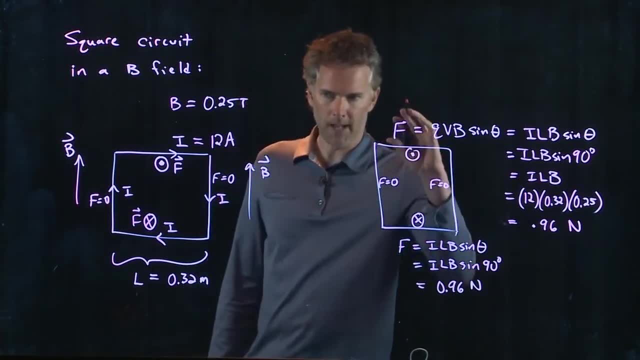 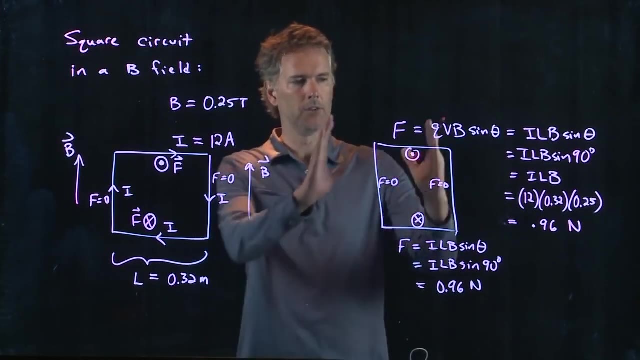 theta, which is 90 degrees, And so we also get 0.96 newtons. Force on the top is exactly the same as a force on the bottom. It means it doesn't move anywhere, but it does rotate, It does twist. 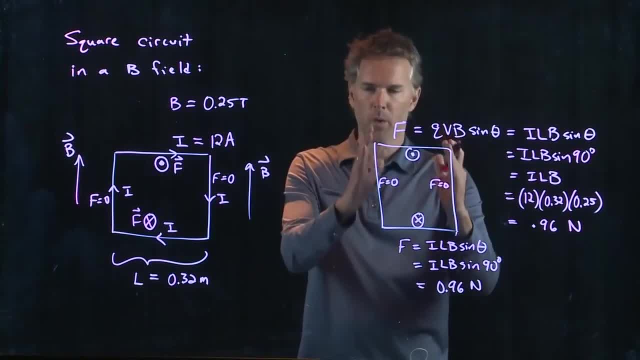 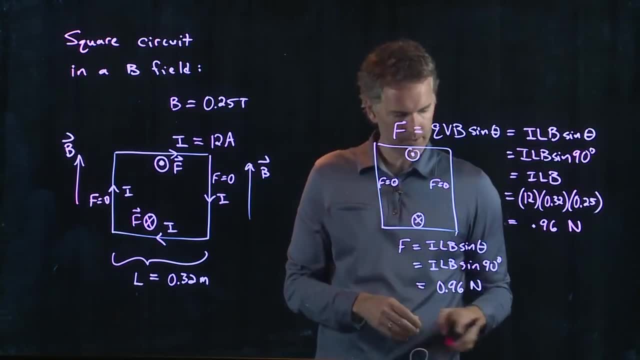 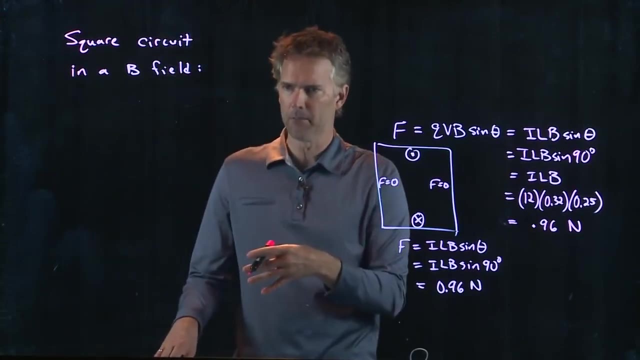 Now, what is that twisting torque? right, When we talk about twist, we talk about TORQ. what is that torque? I know you guys thought you'd forget about TORQ. right, That was so last semester. Do we have to? 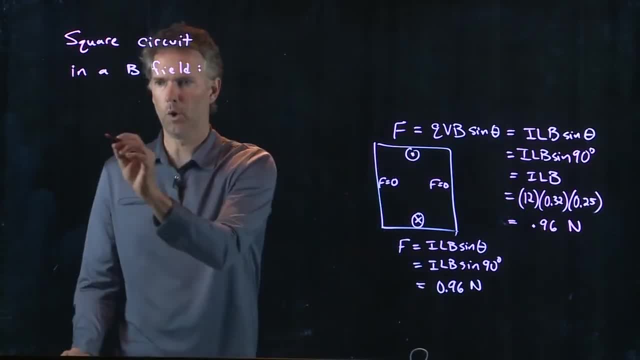 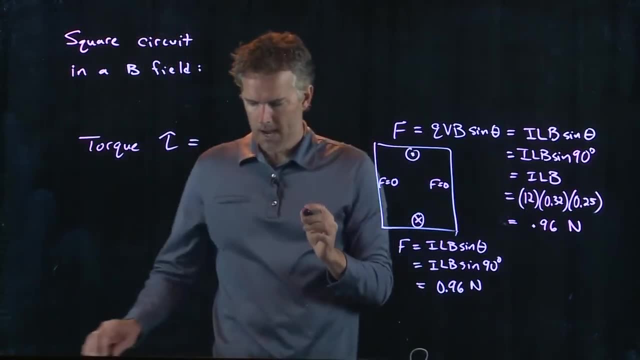 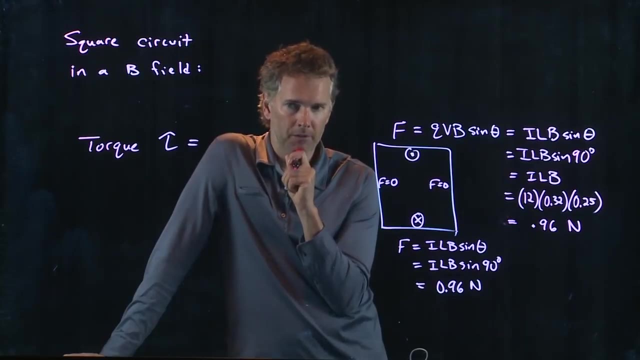 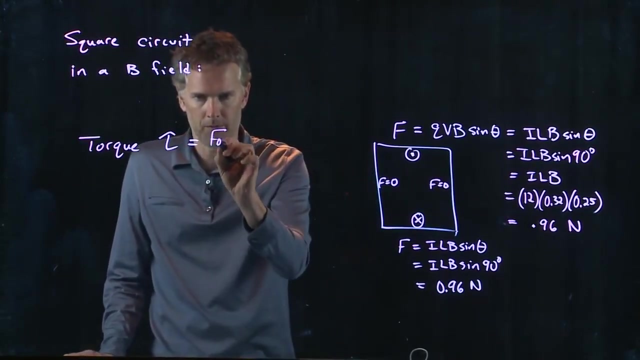 really remember everything from last semester? Yeah, you kind of do. TORQ is written with a tau, Okay, And torque. tau is what? Well, it's force times lever arm. right, Torque is equal to force times lever arm. 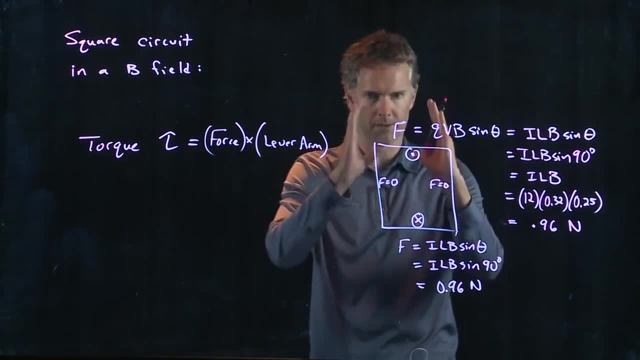 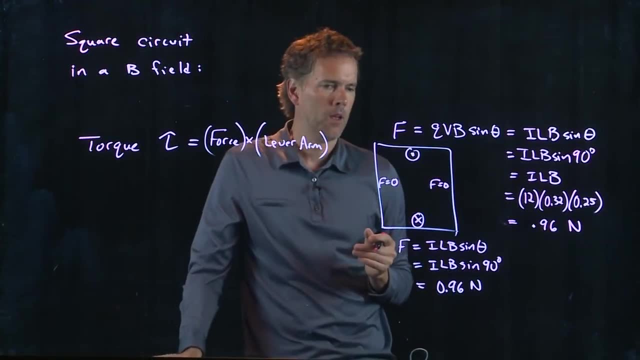 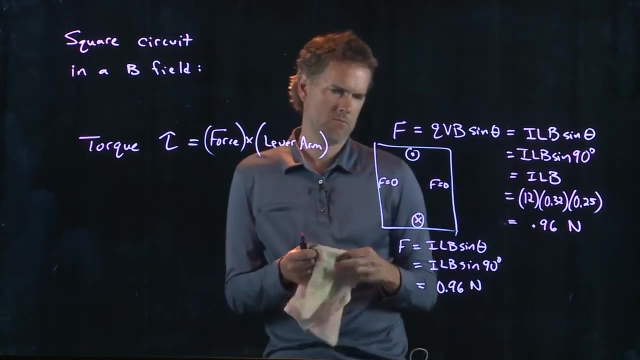 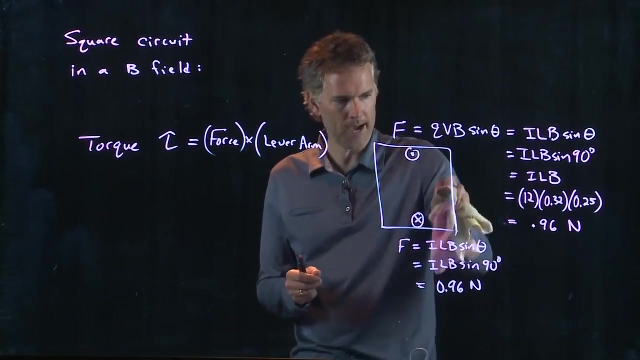 Okay, This whole thing wants to rotate right. The whole square wants to rotate towards you on the top, Away from you on the bottom. What's a good axis of rotation to pick? Well, how about? halfway through Seems like this thing might want to rotate right about its center. 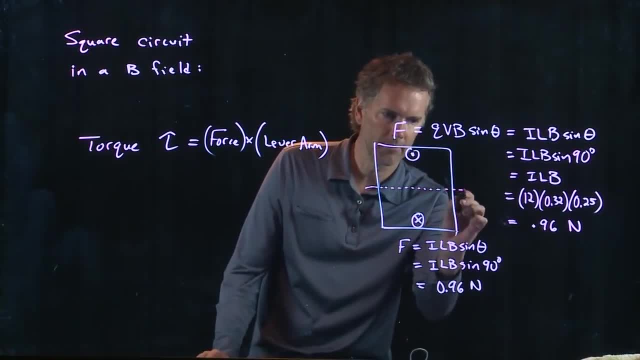 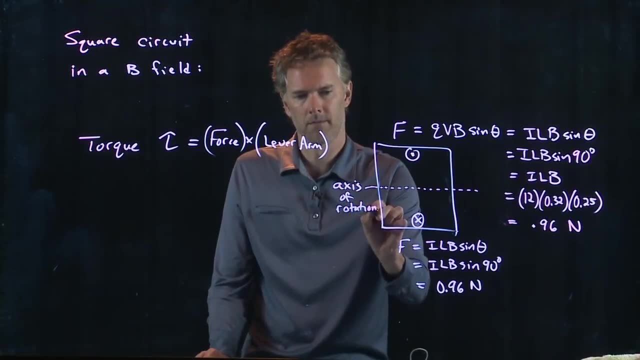 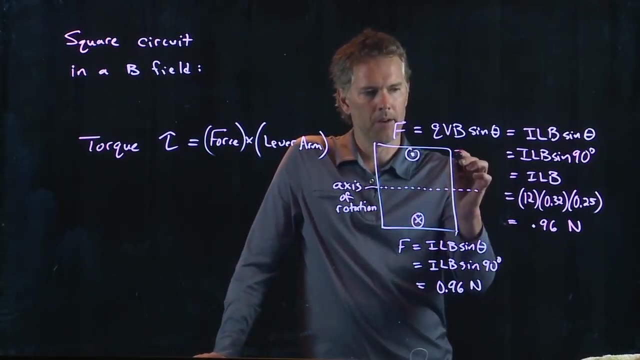 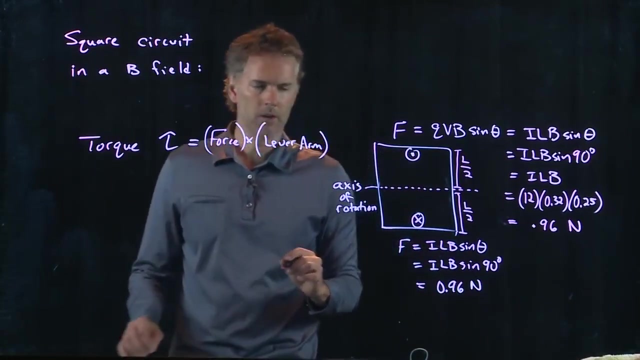 So let's make this our axis of rotation. And if I make that the axis of rotation, then the lever arm here is just L over 2.. And the lever arm on the other side is L over 2.. All right, We want the net torque. 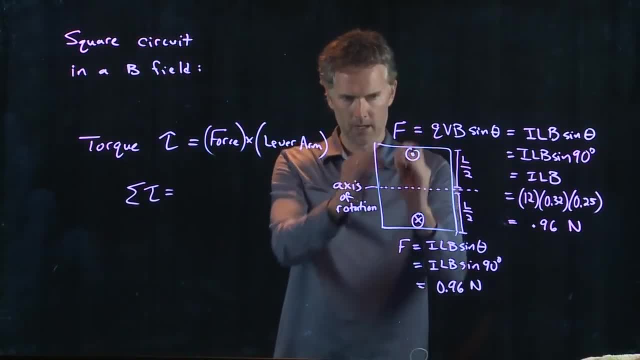 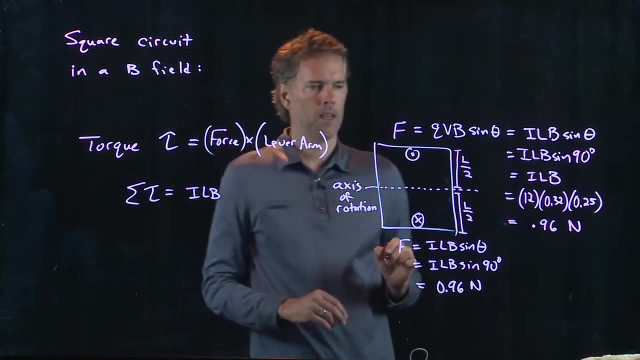 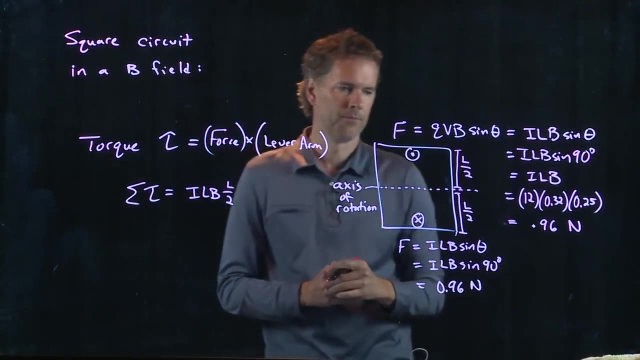 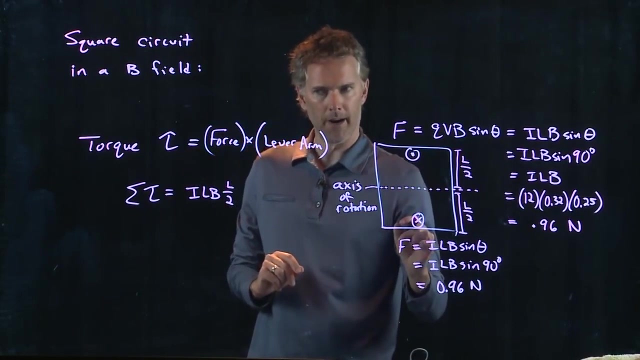 So there is a force on the top side of I, I, I, I times B. There is a lever arm on that top side that is L over 2.. That's the torque due to the top wire, But I also have to add the torque due to the bottom wire. 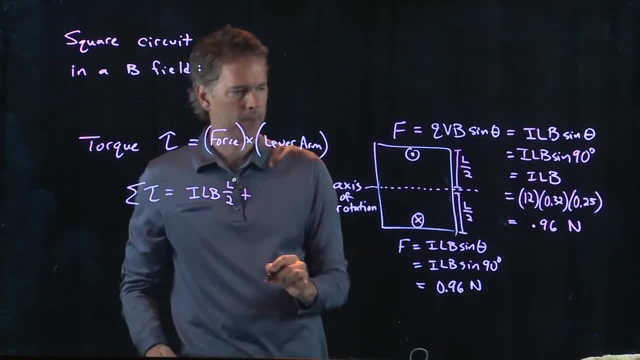 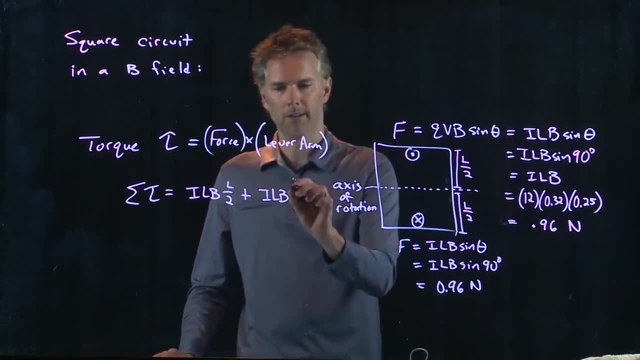 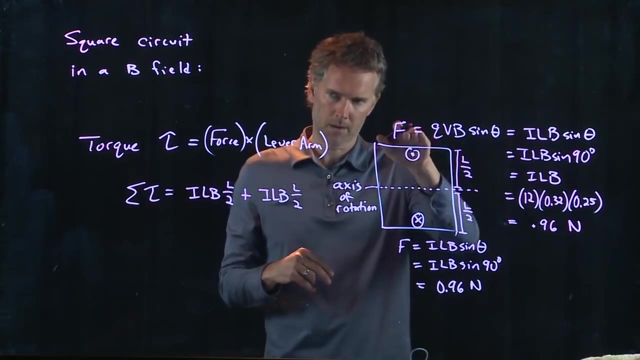 and the torque due to the bottom wire is force. ILB also times the same lever arm because it's trying to rotate it the same way. This force is pushing the top towards you, this one is away from you, and so they're both trying to rotate the object in the same direction. 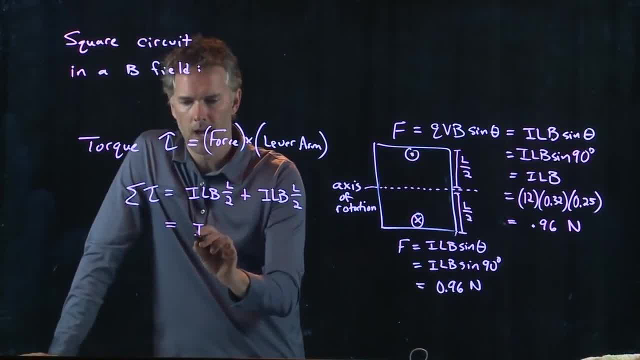 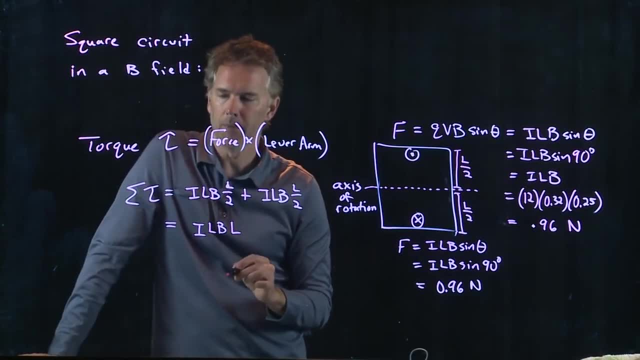 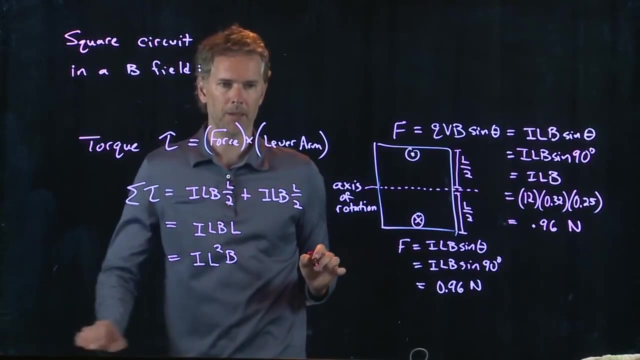 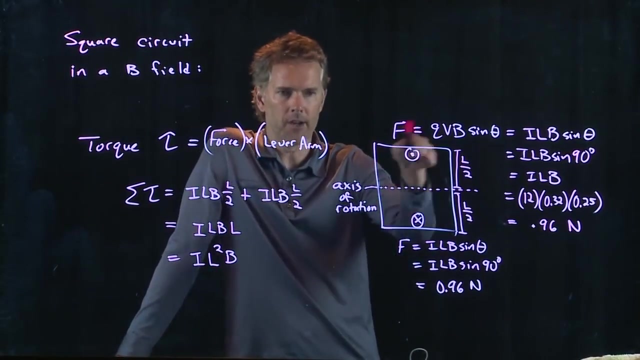 And so now look what happens. We have: I times L times B. I have a half an L and another half an L, and so they combine to give me another one L, And this is IL squared times B. Aha, But L squared. that's just the area of this loop. 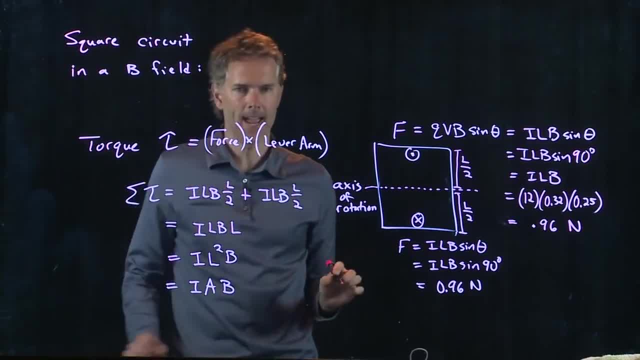 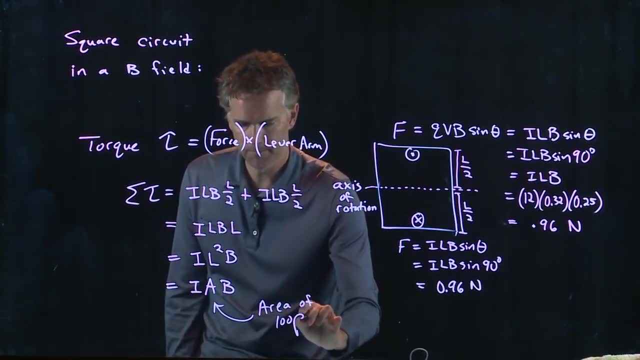 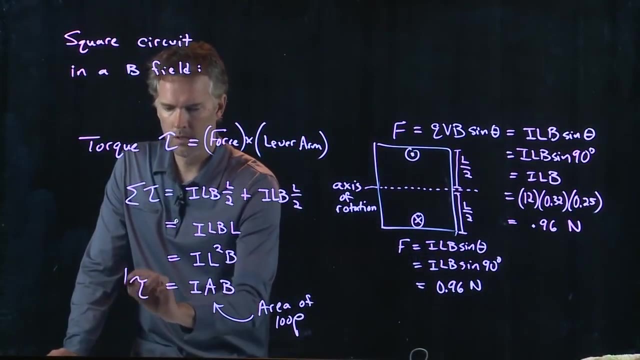 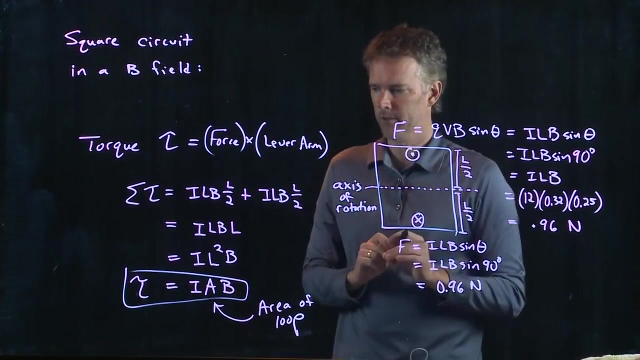 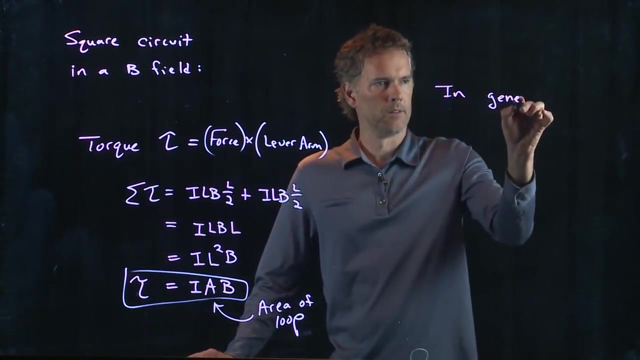 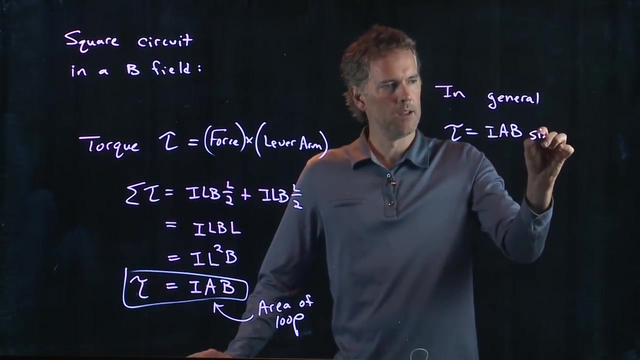 So this whole thing becomes I times A times B, where this thing is the area, And this is torque on a loop if it is at a right angle to the magnetic field. And in general we can write the following: Torque is IAB times the sine of phi. 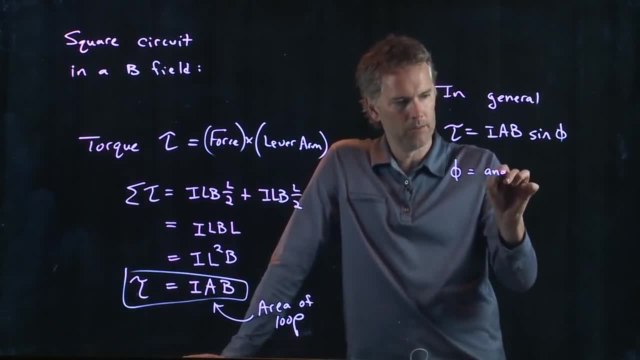 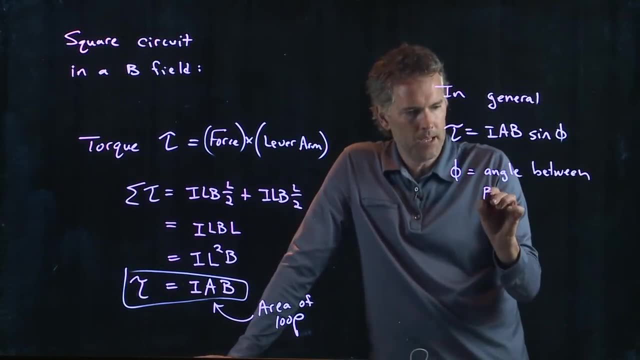 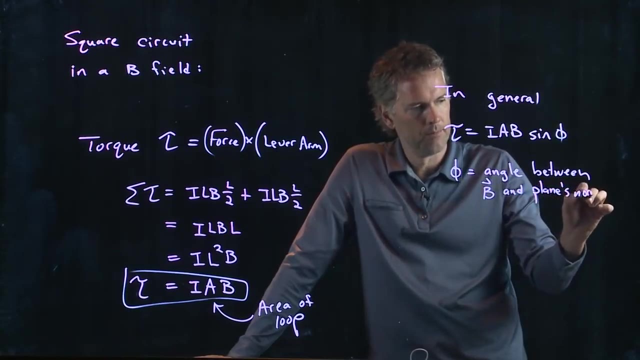 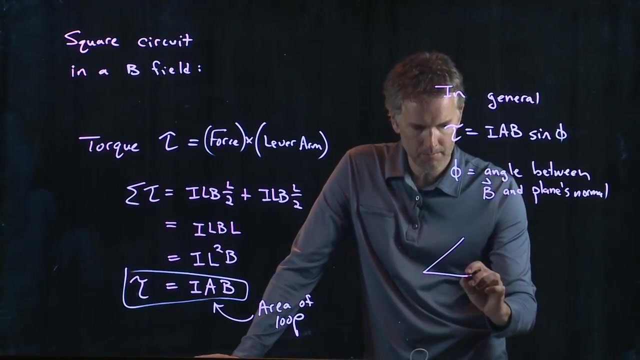 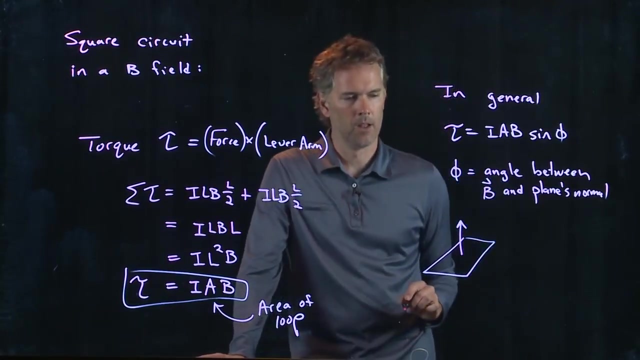 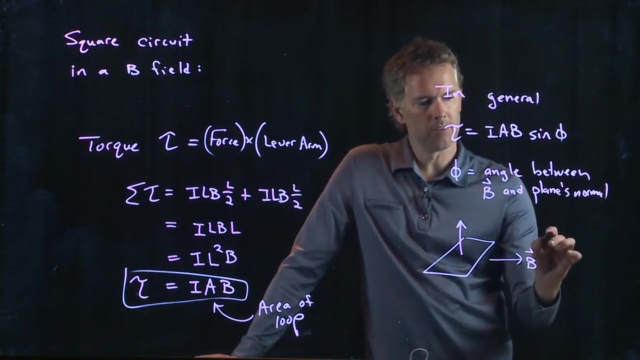 Where phi is the angle between B and the plane's normal. What do we mean by that? Let's say I draw a square loop. okay, the normal would be that. So if the B field is to the right, then phi in this case would equal 90 degrees. 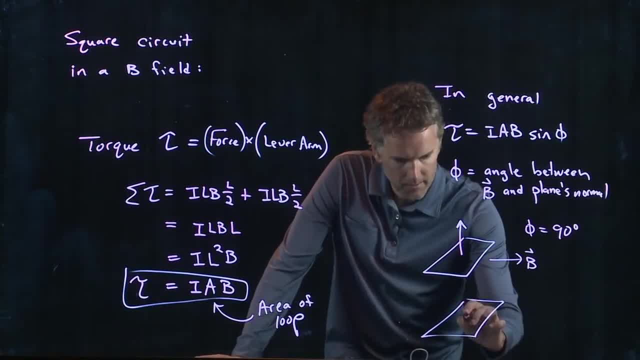 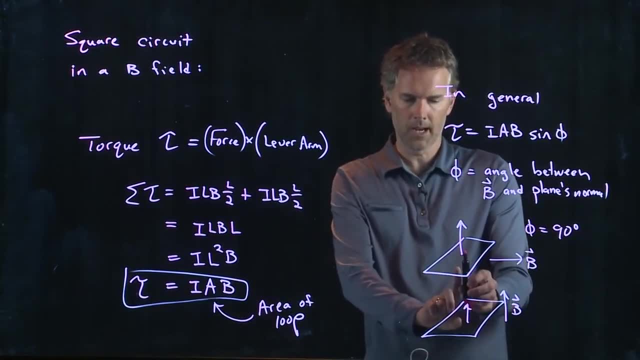 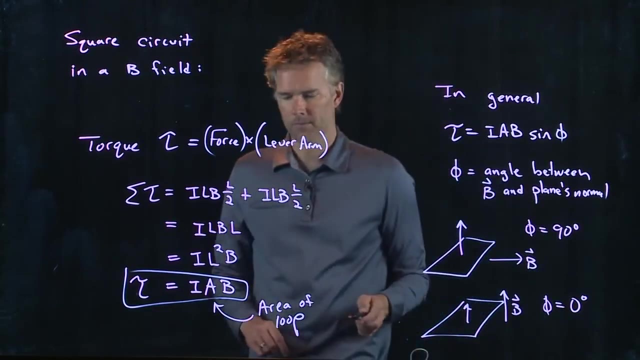 But if I draw it again with the B field going up, then the normal to the plane and B are in the exact same direction. In that case, phi equals zero degrees. Okay, so this phi is between the normal to the loop and the B field.